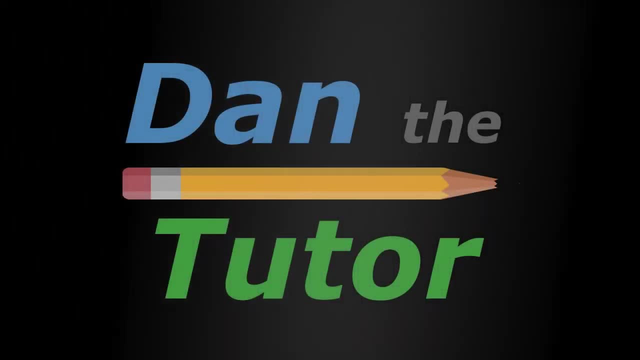 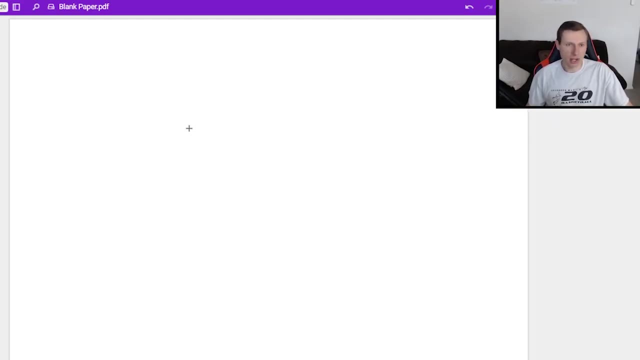 Hello everyone, how's it going? My name is Dan the Tutor. Today we're going to continue our conversation on momentum and we're going to talk about the three types of collisions that you can have in physics, mechanics. Keep in mind that all of these equations are going to use conservation. 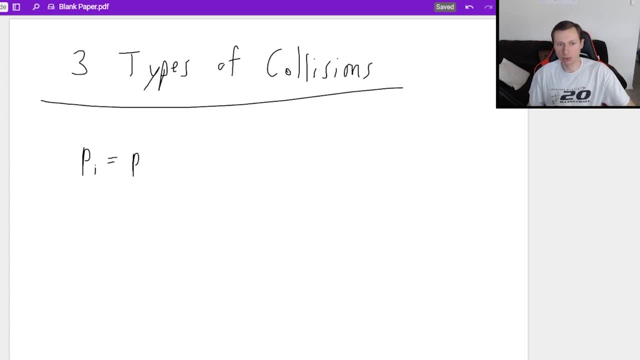 of momentum You have: p initial equals p final. In other words, all the momentum in the first scenario, before the collision, equals all the momentum after the collision. So the three types of collisions are going to be the following: The first kind of collision we have is called elastic. 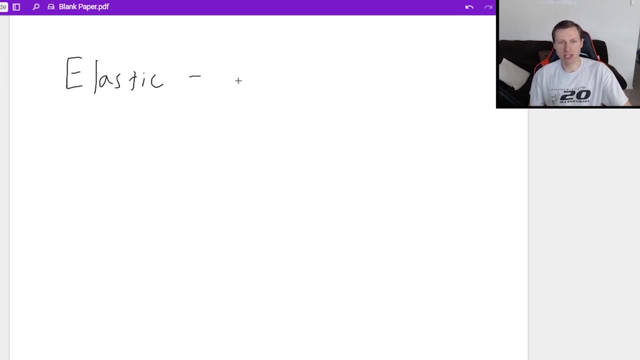 collision, and what's special about this is both momentum and energy are conserved, And so what that means is not only does p initial equal p final, but also the energy total initial is equal to the energy total final. Usually we're talking about kinetic energy here, So like one half mv squared equals one half mv squared, And 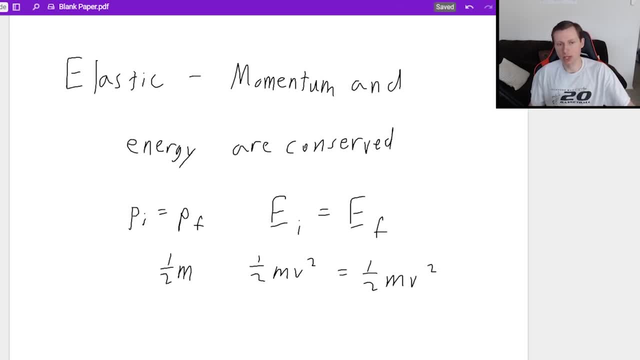 usually we're talking about two objects. So that means one half mass velocity a squared plus one half mass velocity b squared equals the same thing, but for the final scenario. So in other words, energy initial equals energy final, And this is kinetic energy. By the way, elastic collisions do have a special equation because of this. 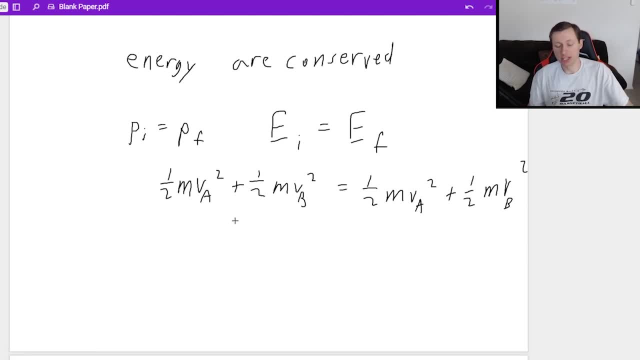 relationship that you can easily find the final velocity of both boxes. So for instance v a, the velocity of the first box or whatever final is equal to parentheses. mass a minus mass b divided by mass a plus mass b. That quantity times v a plus mass b divided by mass a plus mass b: That 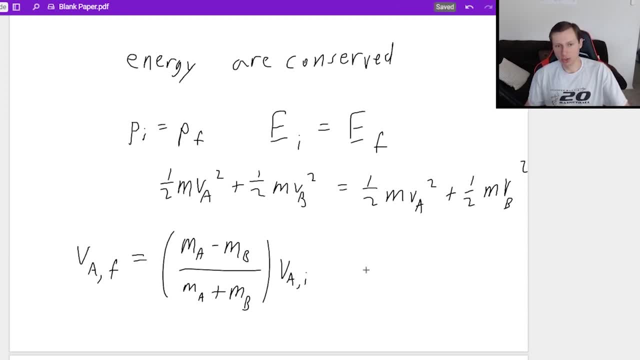 quantity times v a plus mass b, divided by mass a plus mass b, That quantity times v a plus mass b And that's going to be times velocity b initial. And if you happen to get a negative answer for this, that just means it goes to the left. If you get a positive answer, that means it moves to the right. 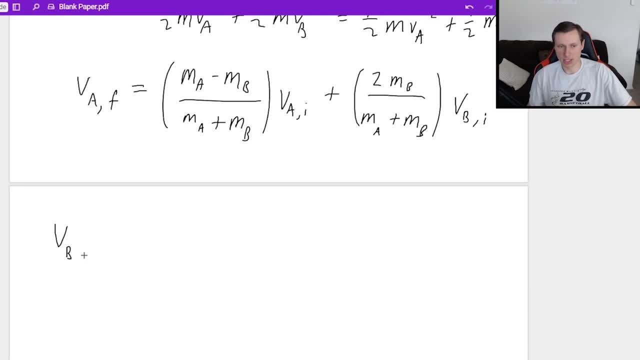 And then for the other box- if you have two boxes colliding- then the velocity for the second object, b, final, it's almost going to be the same as the velocity for the second object. So that's going to be identical to mass a over, mass a plus mass b times velocity a initial plus quantity mass b minus. 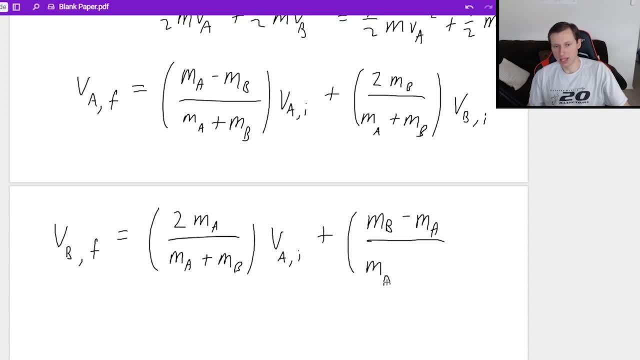 mass a divided by mass a plus mass b, And that's times v b initial. So we have two different equations to find the final velocity of either box. We'll use that today And that's it for elastic collisions. So in other words, we have two different equations to find the final velocity of either box. 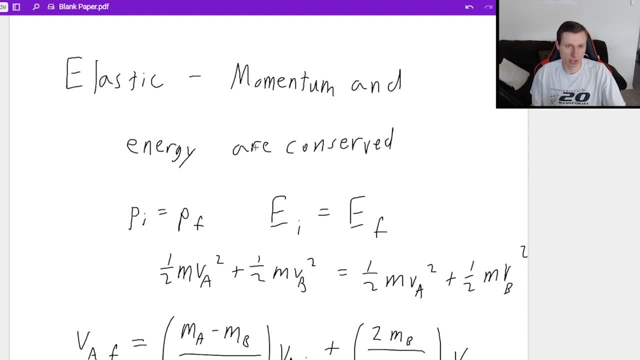 In other words, elastic momentum and energy are both conserved. By the way, for all three of these collisions, momentum is going to be conserved for all three. That's not unique to elastic, And you would use elastic collisions if the problem ever says that the objects collide elastically or if 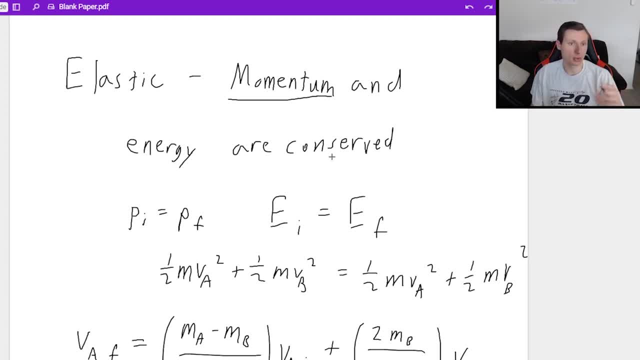 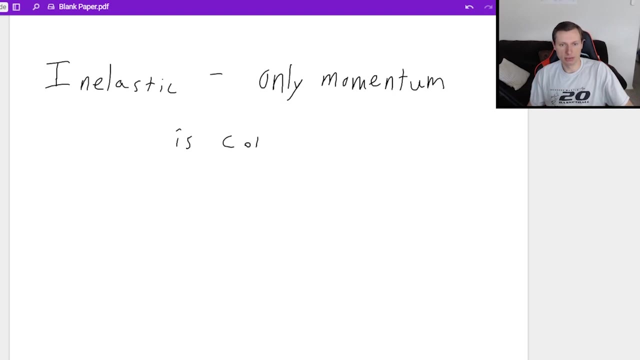 they say: energy is conserved. If they ever say those two words, then you would use elastic. The next kind of collision is called an inelastic collision, And that basically just means that only momentum is conserved, And so the only equation you have is: p initial equals p final. 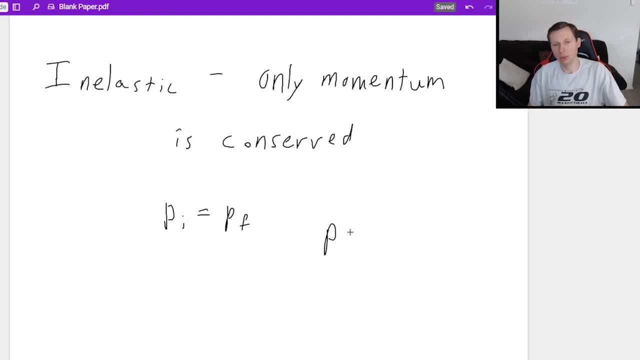 Remember that these p's- I should have mentioned this earlier- p- the equation for momentum p is mass times, velocity, And if I want initial or final I need to add up all the momentums. So I could very well have p1 plus p2 equals p, initial, for instance. That's what I'm trying to. 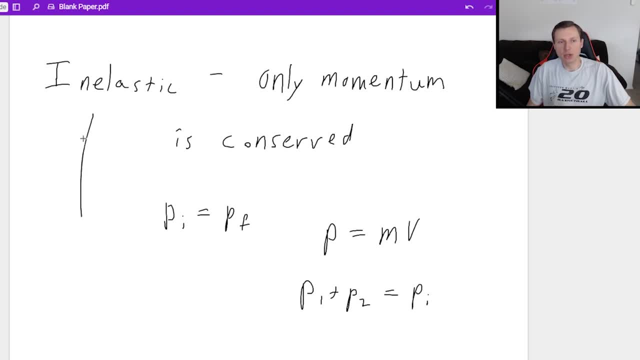 say: And, by the way, when do you use inelastic? They don't even have to tell you it's an inelastic collision. This is the default case. If they don't tell you what kind of collision it is, you assume it's inelastic Because only 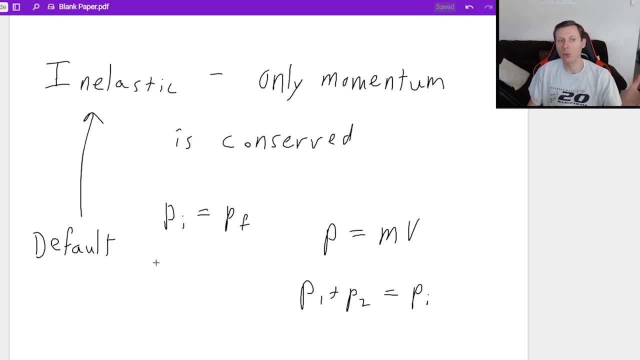 momentum is conserved. you've only got one equation and there's no way you know that energy is conserved, So you can't just assume it's elastic. So we go with inelastic And then the last kind of collision we have is called a perfectly inelastic collision And that basically 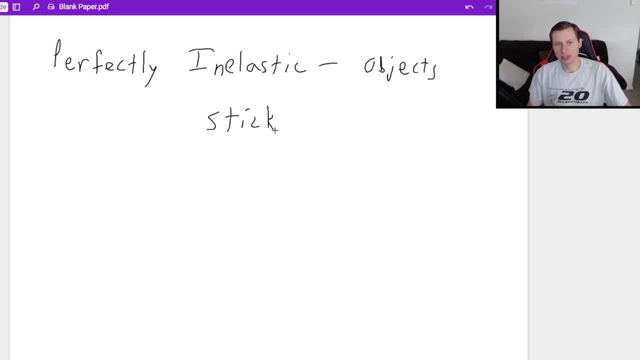 just means that the objects stick together at the end, And what that ends up looking like. for the equation first I write: p initial equals p final again, And what that basically means is that for p final, you're going to add the masses together, because they got stuck together ma plus mb times, whatever their velocity. 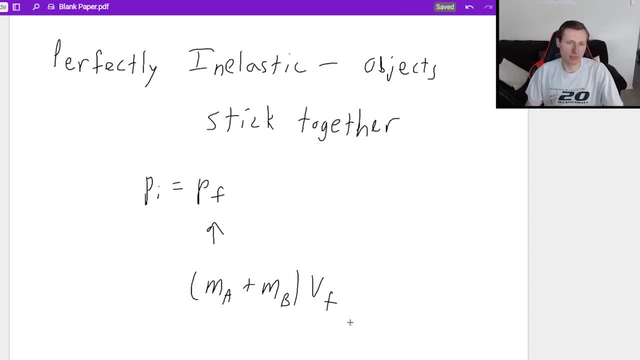 final is: That's how you set up, perfectly inelastic. Obviously, the left side, p initial- is going to change every time, But the right side will be the same every time you add the masses together. Now they're stuck together. So these are the three kinds of collisions. Now let's look at some 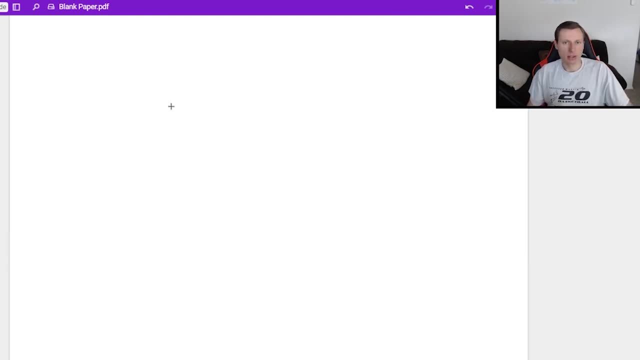 example problems. I have three problems for us today. Here's the first one. Let's say I have two boxes, both with mass, let's say six kilograms, heading towards each other. the first block is going to be heading two meters per second to the right. the other block will be heading eight. 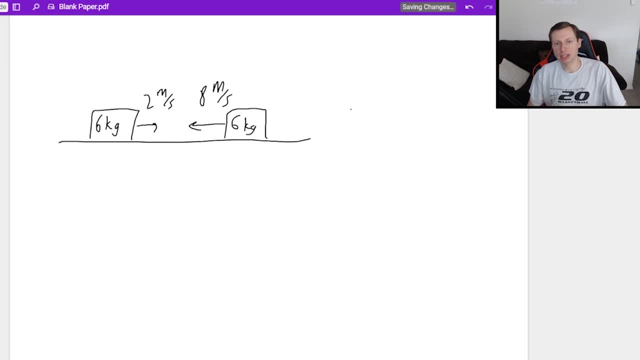 meters per second to the left, And I'm going to say that these boxes collide elastically. In other words, energy is conserved, And I can use that equation I wrote earlier And my question is going to be: what is the velocity of each box after the collision? So this is a pretty straightforward. 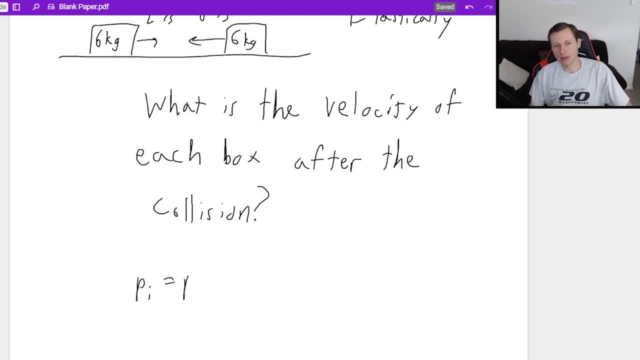 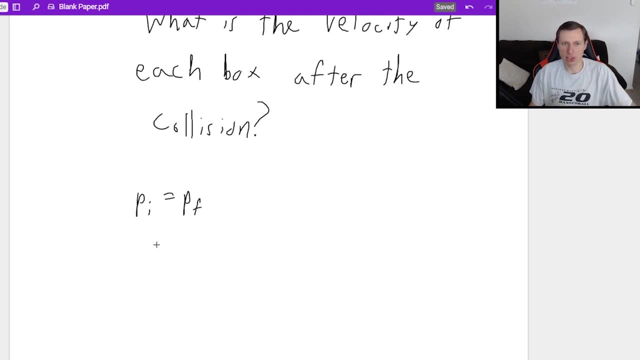 question. I'm not even going to write: p initial equals p final. I mean I can, But the problem you run into is if I set up this equation, p initial is mass times velocity, so six times two for the left one. 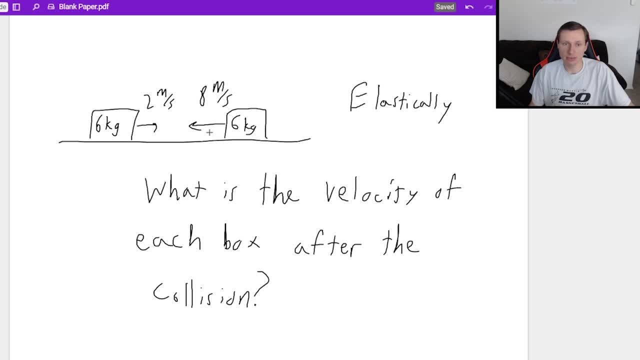 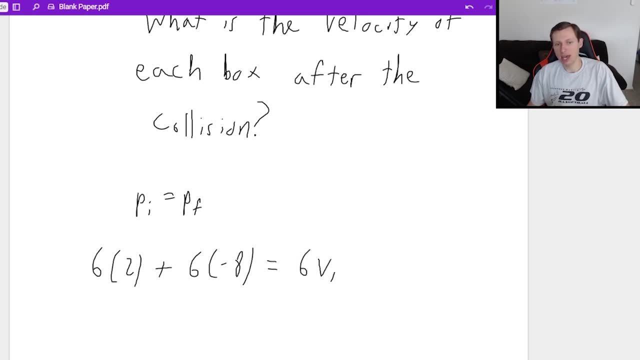 That's momentum for the second one is six times negative eight because it points to the left. So six times negative eight. that part's fine, But p final is six v a plus six v b. both masses are six, But there's no way for me to solve v a and v b right now, So this is not very helpful to us. 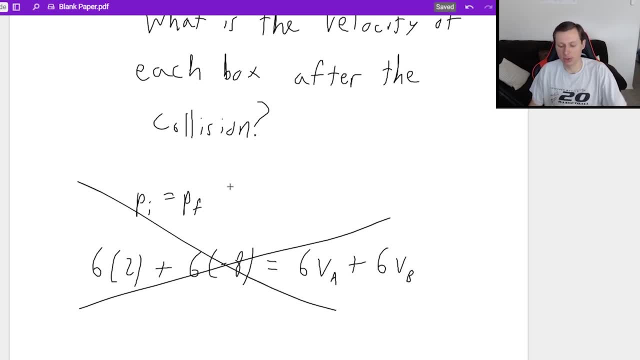 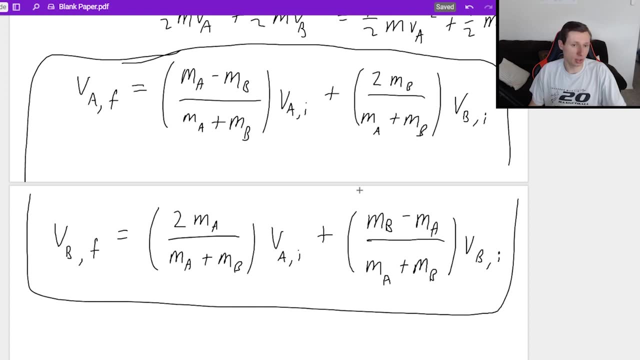 the strategy didn't work. I need to use that equation. I wrote down earlier that long one, the one right here, these two, And I want to tell you that, yes, you can use this equation, it'll work, But there actually is a shortcut for this equation And the shortcut for this problem. 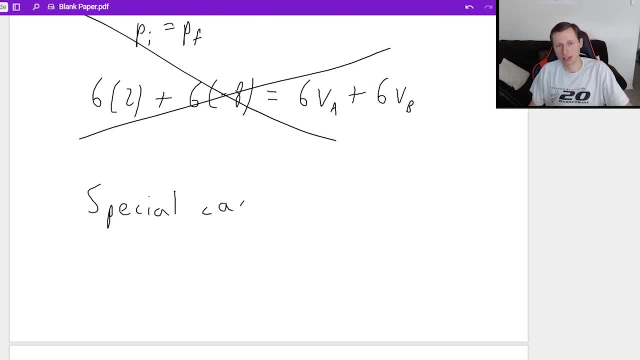 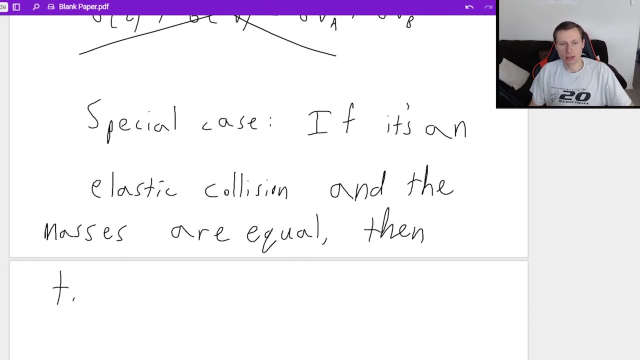 is. there's a special case in the elastic collision. If it's a or an elastic collision and the masses are equal, if you get this, then the final velocities swap. What does that mean? they swap. Well, if initially the six was moving to the right at two, well, I guess they're both six, So that. 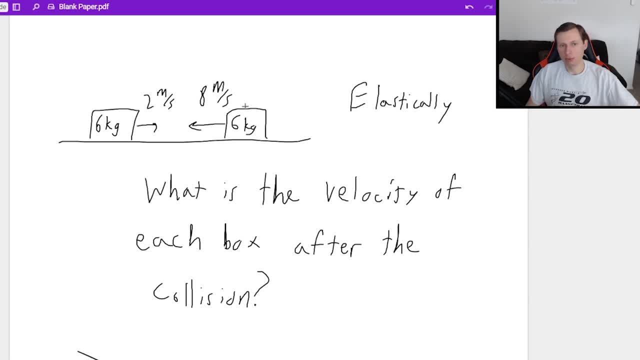 means if the left one moves to the right at two and the right one moves left at eight, then they swap After the collision. I'm literally just going to switch the velocities. So here they are. they just collided And this one is now heading eight to the left And the other one is now 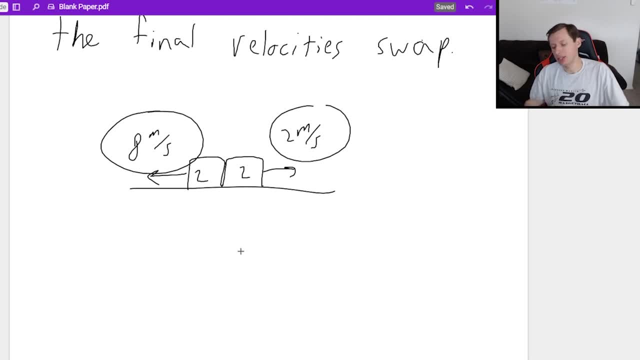 heading two to the right And we're done. And again, this is a special case of the elastic collision, when the masses are equal to each other. And should you memorize that, I would. it's not that hard And it will probably show up at some. 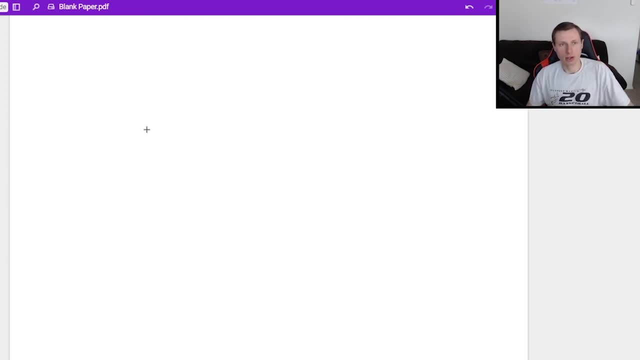 point on your quiz or test. So that's it for the first one. For the next problem, we're going to have a little fender bender. So we've got two cars here. we've got car A and car B. Car A is: 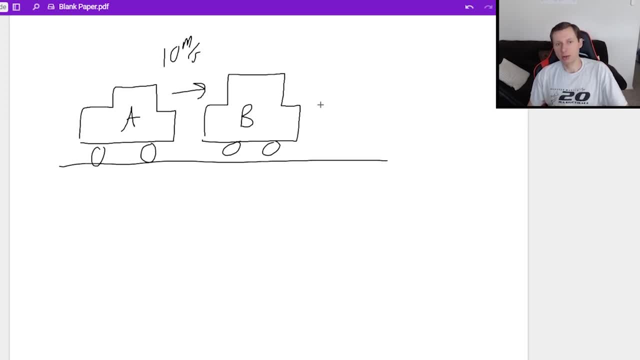 moving to the right at 10 meters per second And car B is also moving to the right, but only at two meters per second. Since car A is moving faster, they are going to get into a collision there. Don't worry, they have good insurance. Don't worry about that. I'll say the mass of car A is 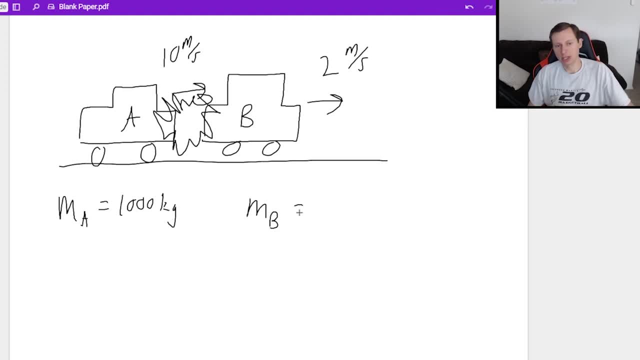 1000 kilograms And the mass of car B. let's say it's a truck and say it is 2000 kilograms. I have no idea how much a car weighs, especially not in kilograms. So as far as I'm concerned, these are: 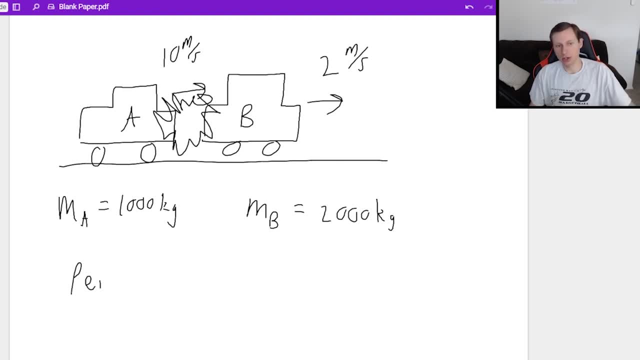 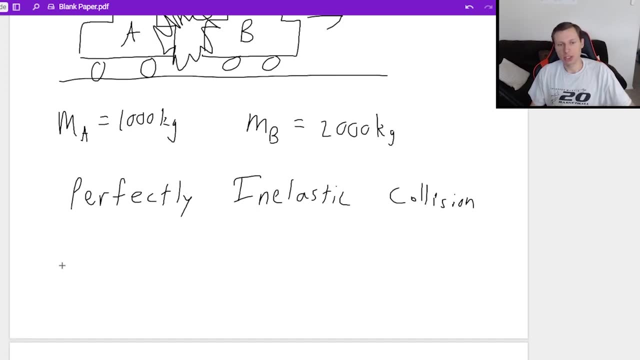 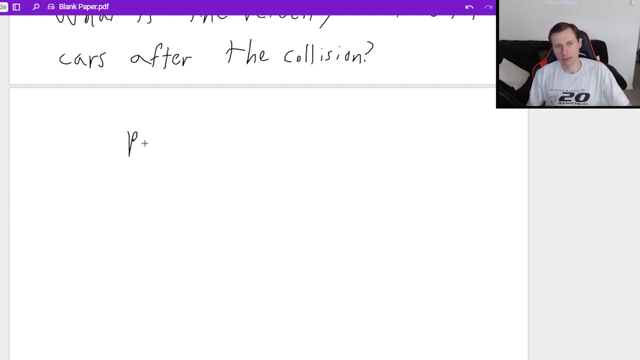 good numbers And let's say, during the collision they undergo a perfectly inelastic collision And my question is going to be: what is the velocity of both cars after the collision? So I just set up my equation for perfectly inelastic collisions: P initial equals P final, where I know the objects are going to stick. 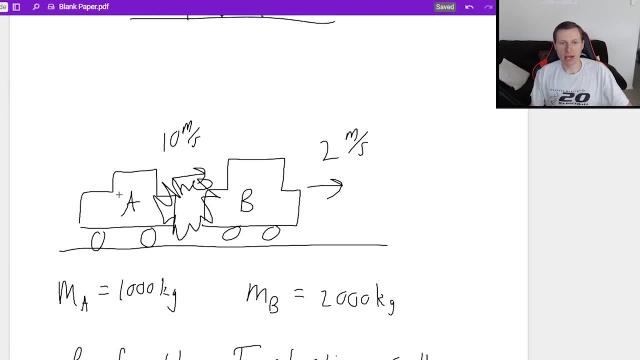 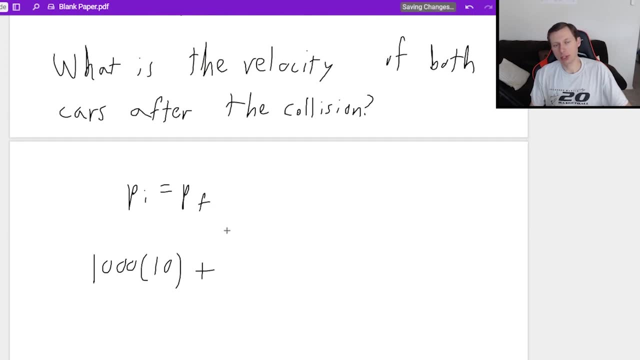 together at the end. So for P initial got car A which has a momentum of mass times, velocity 1000 times 10,, 1000 times 10.. And then plus the velocity of car B, which is 2000 times 2.. And 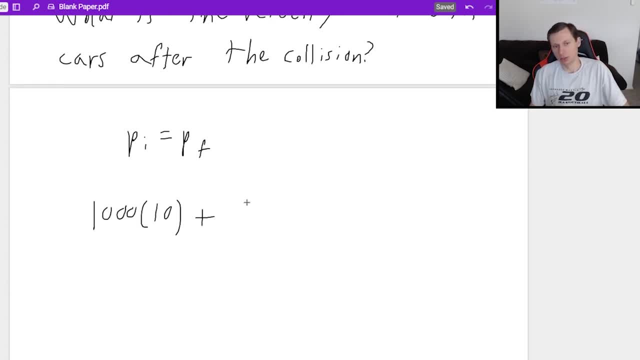 they're both positive since they point in the right direction. And then plus the velocity of car B, which is 2000 times 10.. And they're both positive since they point in the same direction, to the right. So 2000 times 2, that is equal to P final, which is the masses added together, 1000 plus 2000,. 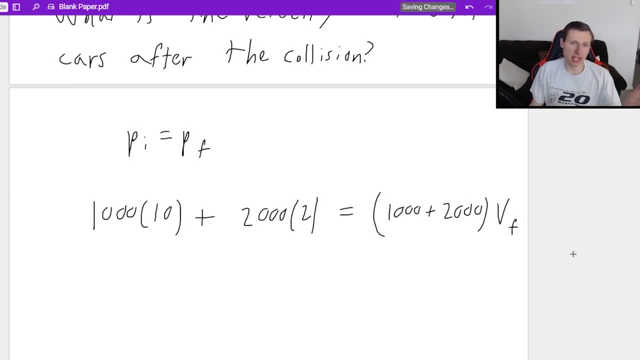 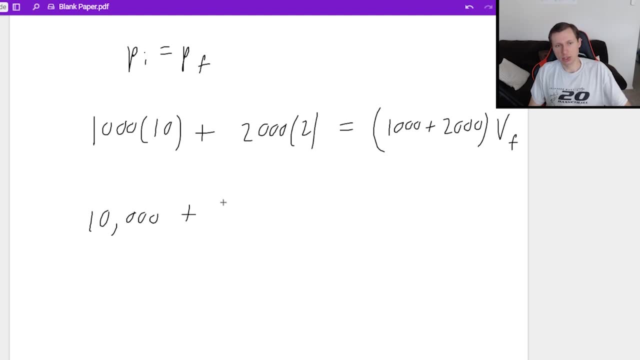 times their velocity final And they're going to have the same velocity because now they're stuck together after the collision. So 1000 times 10 is 10,000, plus 2000 times 2 is 4000. That equals. 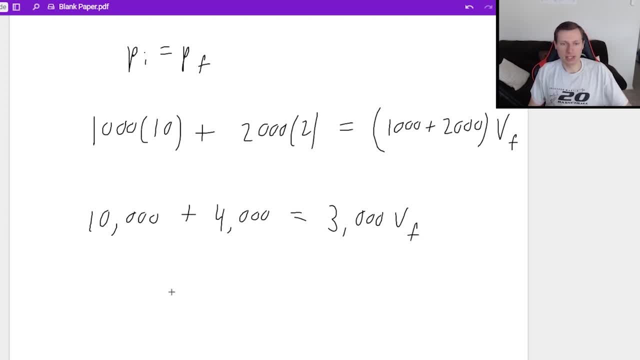 3000 V final. Add the 10 and the 4, 14,000.. Equals 3000 V final. And then I just divide by 3000. And I'll get a final speed of 4.67 meters per second. And that is the velocity of both cars. 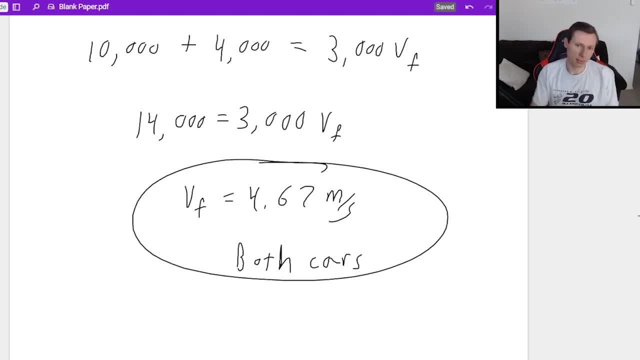 because they're moving together. So that's going to do it for that problem. And now the last problem we have. it's a fun one. I'm going to give you a scenario, So I'll give you a before and after picture. 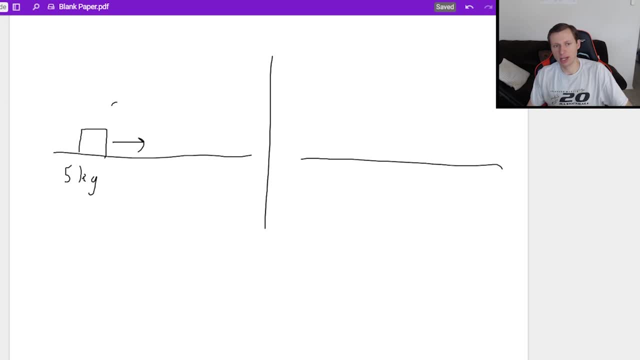 Ideally, a 5 kilogram mass is moving to the right at 2 meters per second And a 10 kilogram mass is at rest After the collision. the 5 kilogram mass is going to be moving backwards now at 2. 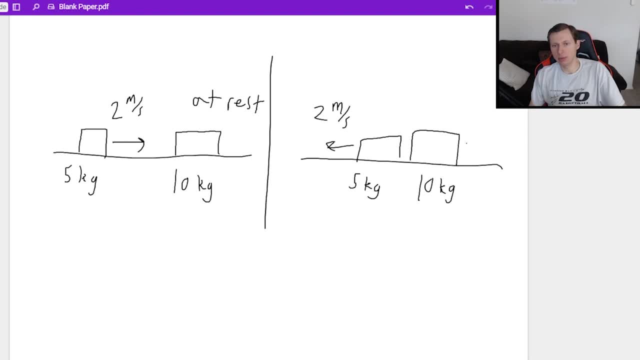 meters per second, And the 10 kilogram mass is going to be moving forward, but at an unknown velocity. I have two questions for this problem. Number one: what is the velocity of the 10 kilogram mass? And my second question is going to be: what kind of collision is this, Which? that's an interesting 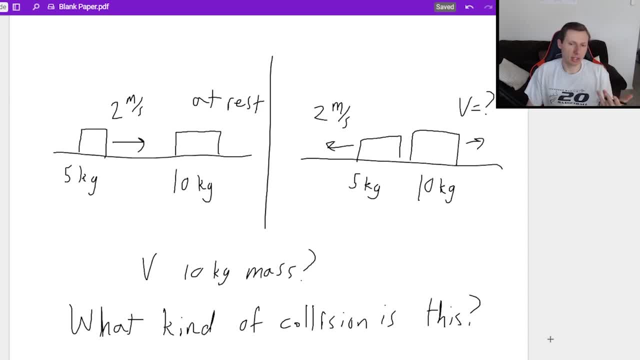 question. How would I answer that? So remember, there's three kinds of collisions: elastic, inelastic and perfectly inelastic. You know, perfectly inelastic is when the objects stick together, which is clearly not happening here. The other one's rebounding in the opposite direction. 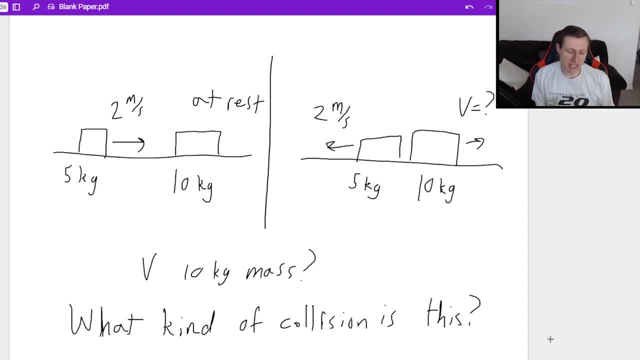 So it's not perfectly inelastic, which means it's either elastic or inelastic. And the way we tell is: well, is energy conserved? If energy is conserved, then it's going to be elastic. If it's not, then it's going to be inelastic. And so here's what I'm going to say. First, need to find. 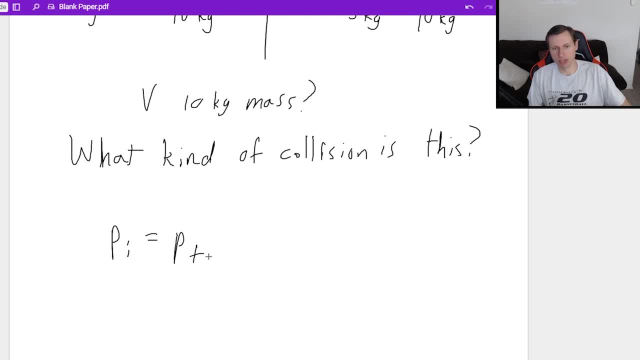 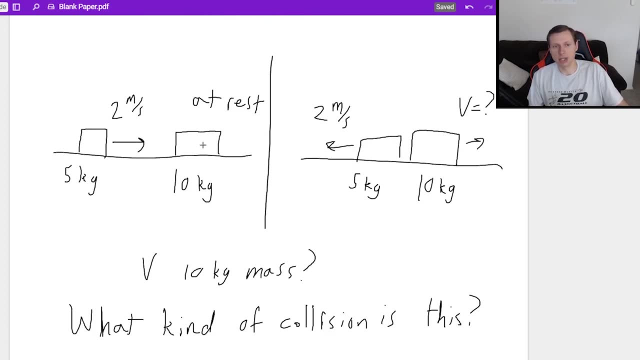 that velocity- So that just involves P initial- equals P final. simple equation: P initial is 2 times 5, because that's the momentum of the first one, plus the momentum of the 10 is 10 times 0, because its velocity is at rest. That equals P final, which for the 5 kilogram mass is 5 times. 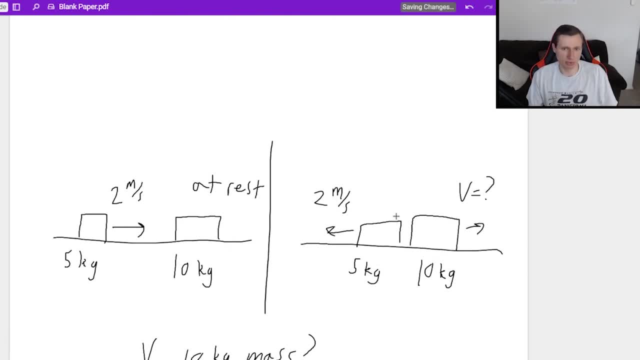 negative 2.. Don't forget that negative because it moves to the left now And then, plus the mass, 10 times its velocity, V, which is what I'm solving for. So I start plugging in: 5 times 2 is 10,. 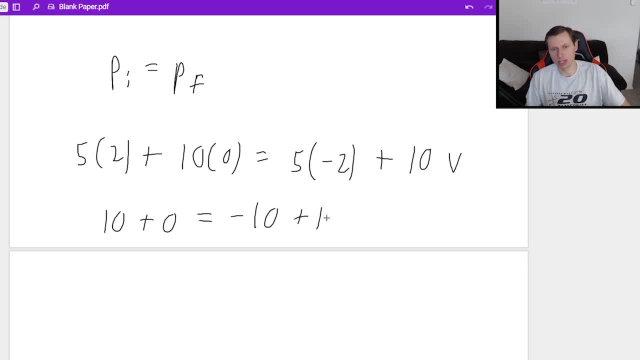 plus 0 equals negative. 10 plus 10V. I need to add 10 to both sides here. Looks like I'm going to get 20 equals 10V. Just divide both sides by 2.. V equals 2 meters per second, And that's positive. 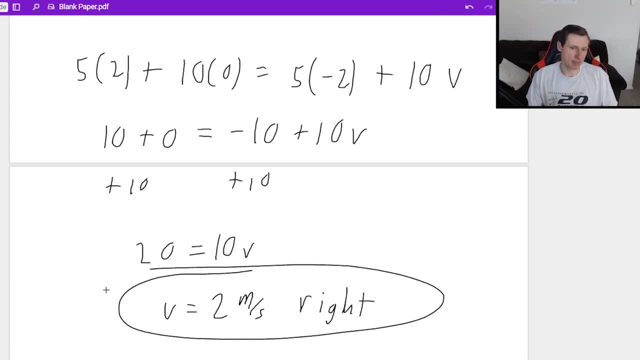 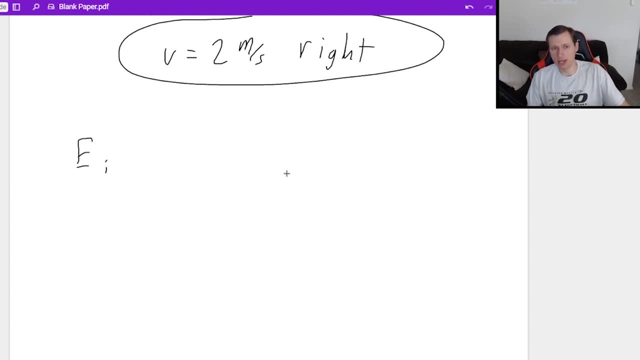 which means it points to the right. So there's my velocity. Now I just need to find whether or not energy is conserved. So that means E initial First. I'm going to do that and then we'll find E final. But energy initial is 1 half. 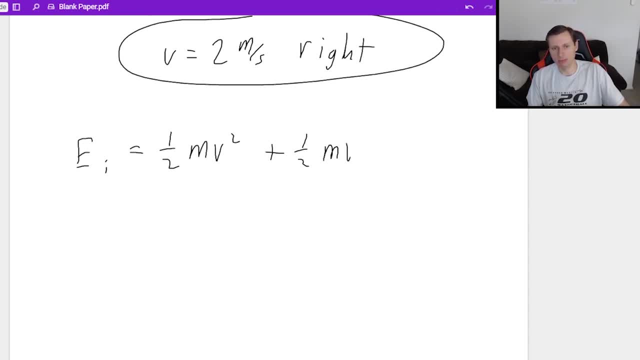 MV squared for the first box, plus 1 half MV squared for the second box, which is going to be 1 half. Mass is 5 for the first one. Its velocity is 2, positive 2.. I'll square it And then the 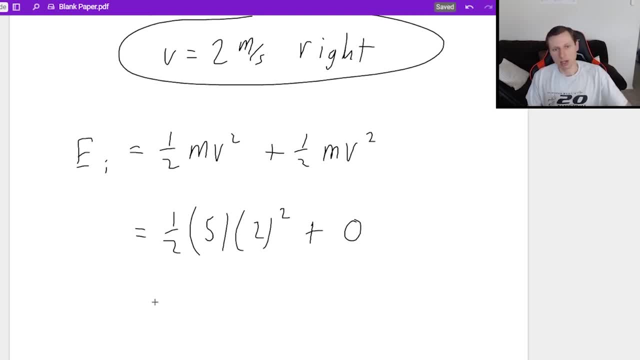 energy for the second one is just 0, because the velocity is 0. So that's going to give me- if I plug this in my calculator or you can just do it in your head, you get 10 joules of energy. Now that's energy, initial, And so if it's elastic, 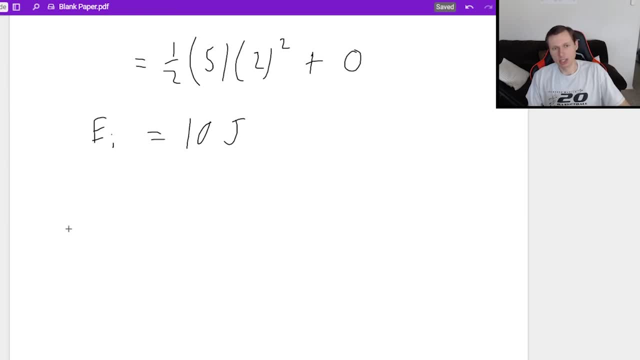 then my energy final will be 10 joules. So let's see what the final energy is now. So for that one, remember, it's 2 meters per second left And this one we just discovered to be 2 meters per second to the right. So it's going to be 1 half mass, 5 velocity negative 2.